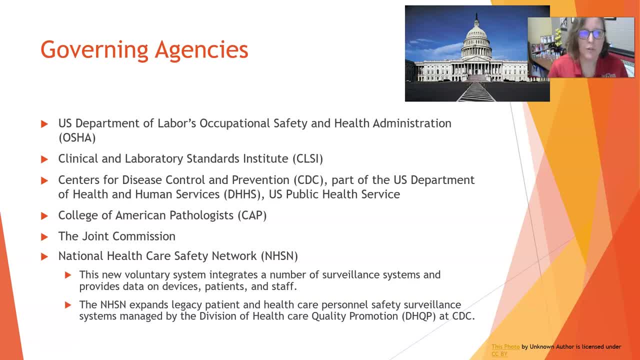 that apply to the lab more specifically, of course, are the US Department of Labor's OSHA, so Occupational Safety and Health Administration, the Clinical Laboratory Standards Institute, so that's more lab specific, also known as CLSI. So they put out the standards that you need to go. 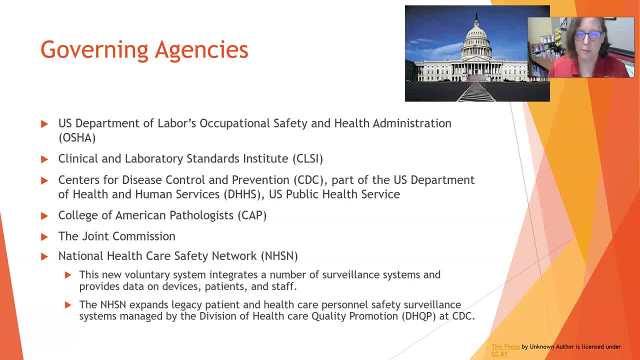 by to have a high quality lab with high quality patient care and high quality results. Then we have the Centers for Disease Control and Prevention, which is part of the US Department of Health and Human Services, and also the US Public Health Service. So the US Public Health Service, or US, 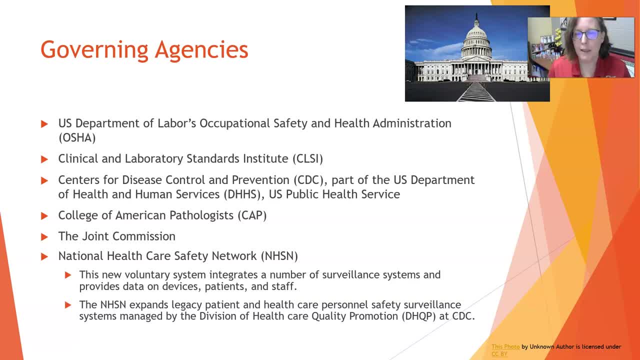 Public Health Service Corps is a corps of uniformed personnel that is dedicated to health, and they're embedded in governmental agencies such as the CDC, but not only in the CDC, They're all over the place. Next we have the College of American Pathologists, or CAP, So that one is voluntary organizations. 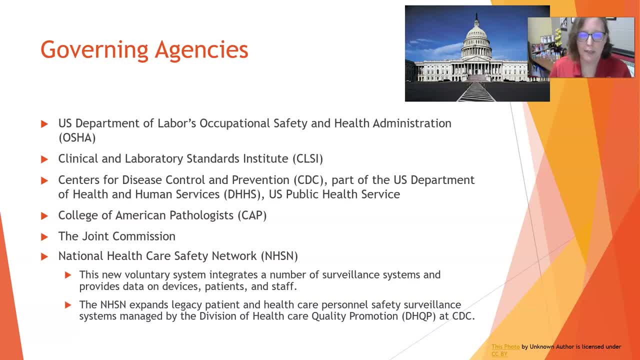 so labs can choose to be accredited by CAP, and if they are accredited by CAP they have to abide by all the CAP standards. Then there's the Joint Commission. That one's not optional Joint Commission comes in, inspects hospitals and they accredit those hospitals in some of the things that 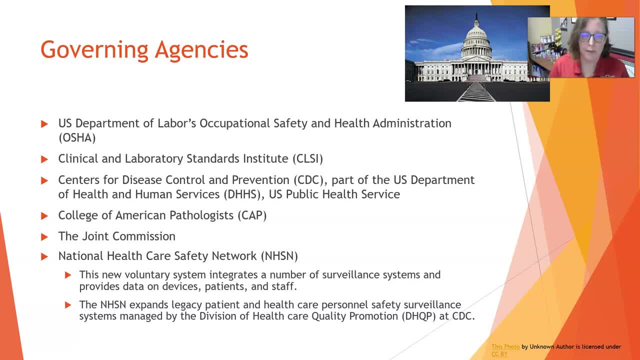 they'll look at and come in the lab and look at, are going to be more safety-oriented. Then there's also the National Healthcare Safety Network. So this is a new voluntary system. It integrates a number of surveillance systems all in one place and it gives you data on devices, patients and 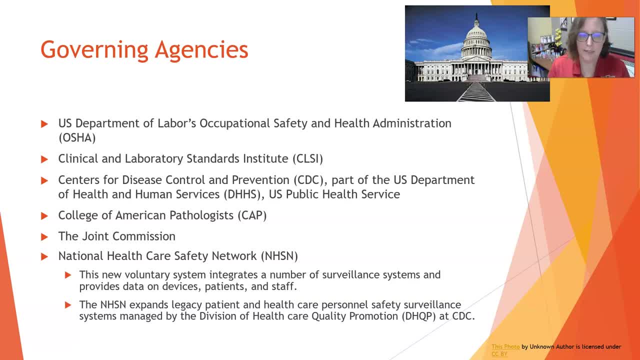 staff, And so it expands legacy patient and healthcare personnel safety surveillance systems that are managed by the Division of Healthcare Safety and Safety. And then there's the National Healthcare Quality and Promotion at the CDC, So it is a branch of the CDC now, and you can go on. 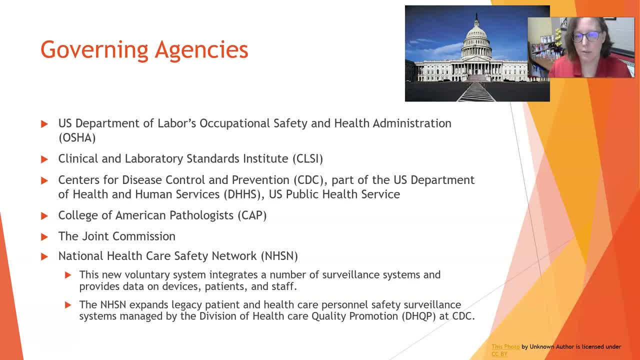 there, And some of the things that they deal with is, you know, it's one report- reports from institutions to the safety network, but then also like how to deal with different things, So especially hospital-acquired infections, such as you know, surgically acquired infections. 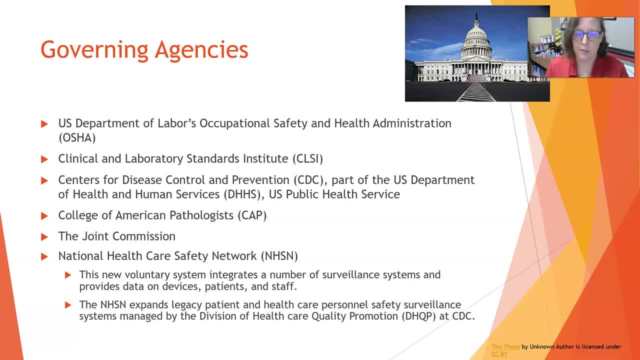 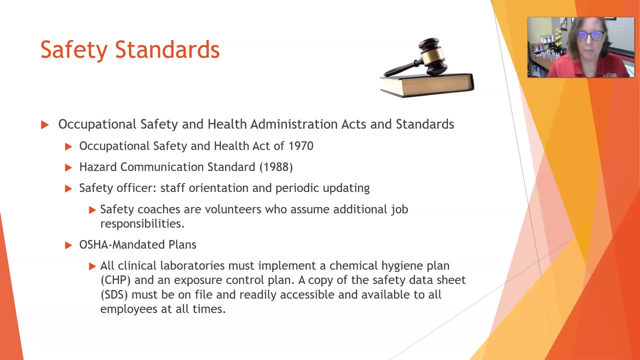 ventilator-associated pneumonias, antibiotic-resistant conditions, etc. So you can go, you can look them up and go in and you can look up by facility and then see what kind of protocols and standards they have for you. So as far as safety standards, we have the OSHA acts and standards. So OSHA was established in. 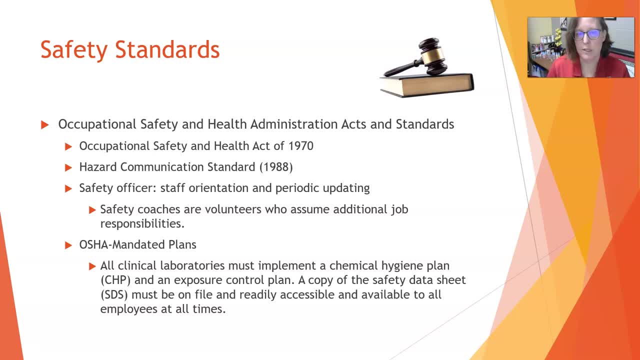 1970.. So that's what started it And that was obviously to increase workplace safety across industry and across all over. This is beyond healthcare. This is everywhere in the United States. So it's been around. since we've been in the United States, I think, I think it's been around. 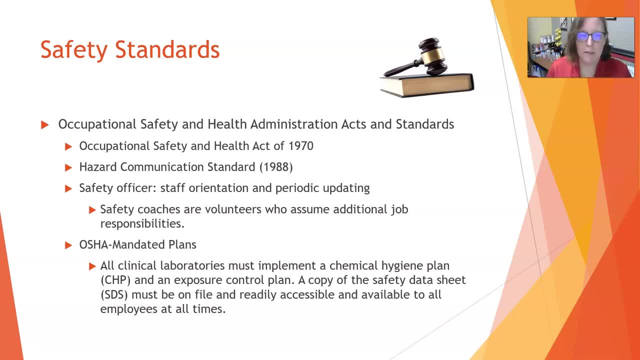 I think it's been around the United States. I think it's been around the United States, I think it's been- of States where people are employed. The next most impactful act was going to be the hazard communication standard, which was passed in 1988, which I'm going to cover here in just a second. 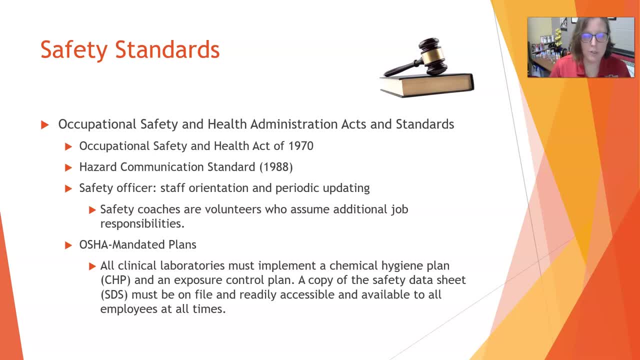 Also part of OSHA. there should be a safety officer at each workplace and they are responsible for conducting the staff orientation part that is going to be dealing with safety and safely doing the job And then, of course, periodic updating for the entire staff of the facility Safety. 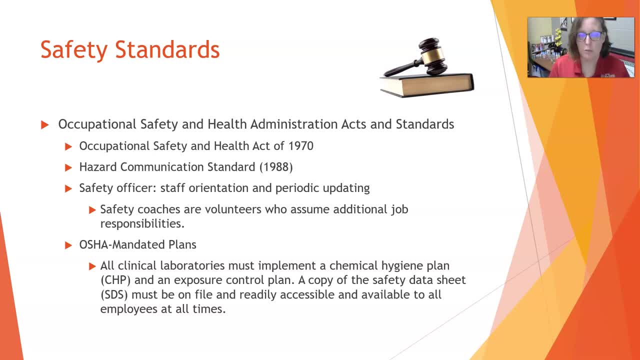 coaches are volunteers who assume additional job responsibilities on top of their own. So that would be. you know, you could be a nurse and a safety coach, you could be a lab tech and a safety coach, And then you would be the go-to person in your specific area or department when safety. 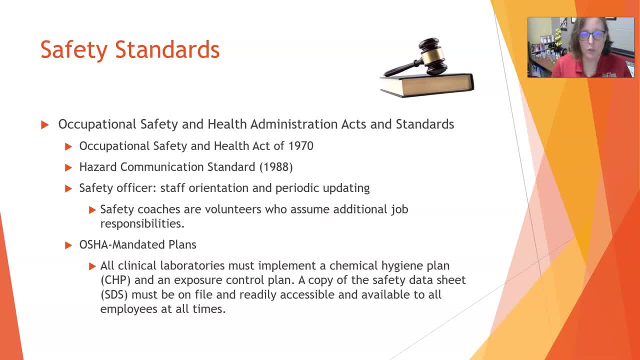 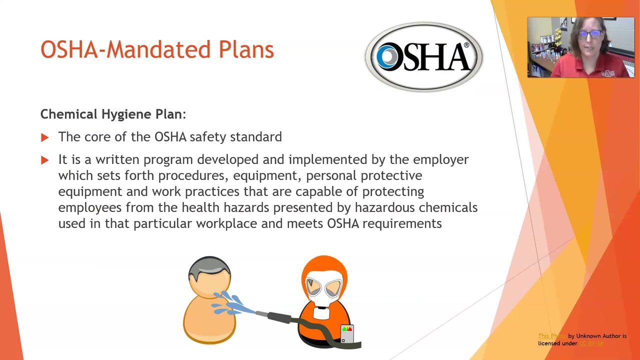 concerns arise, And then there are some OSHA mechanisms. So we're going to cover what all that is here in just a second. So let's start with a chemical hygiene plan. It is the core of the OSHA safety standard. What is it? So it's a written program. 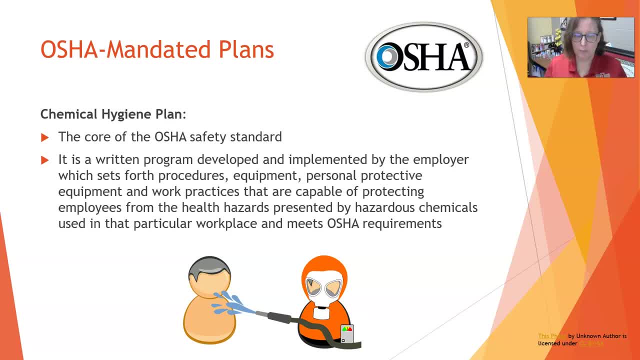 that is developed and implemented by the employer, And so this would be developed by each individual lab has to do this, okay, And it sets forth procedures, equipment, personal protective equipment, work practices, et cetera, that are capable of protecting the employees from. 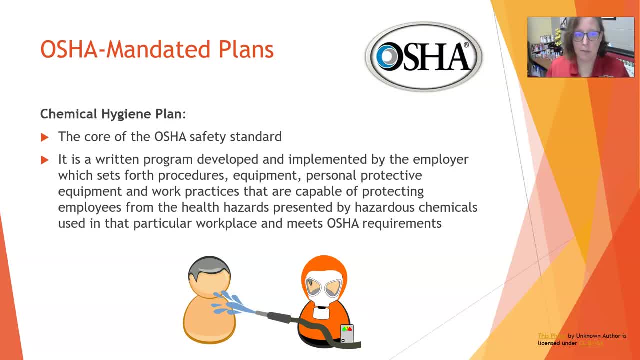 health hazards that are due to hazardous chemicals in that particular workplace and meets OSHA requirements. And so in the lab there are a lot of reagents, there are a lot of chemicals that we deal with, And so part of the chemical hygiene plan is: 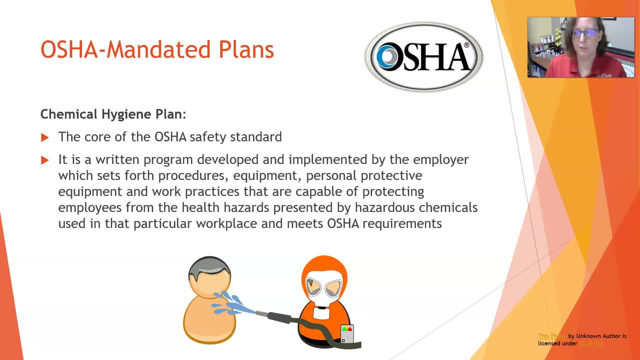 you know how do you handle them, These chemicals? do you have to have a fume hood? Do you have to have a mask? Do you have to have gloves? Are you concerned about it catching fire, about it exploding? Are you concerned about breathing in the fumes? Are you concerned with like exposure? 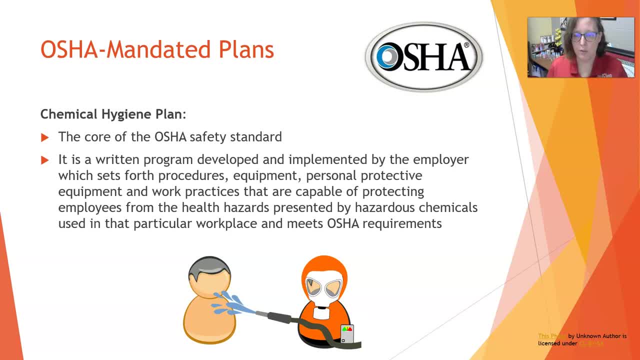 to the skin And you know what's the best way to handle it so you don't hurt yourself. And then, if you do get exposed, like, how do you handle it? And then you know what's the best way to. 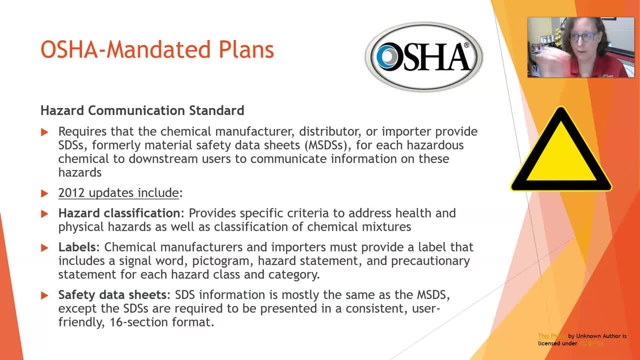 handle it? How do you deal with it? What do you do? And this is for every chemical that is located in that particular lab. So the hazard communication standards. so that was the 1988 update to the OSHA Act. It requires that the chemical manufacturer, distributor or importer 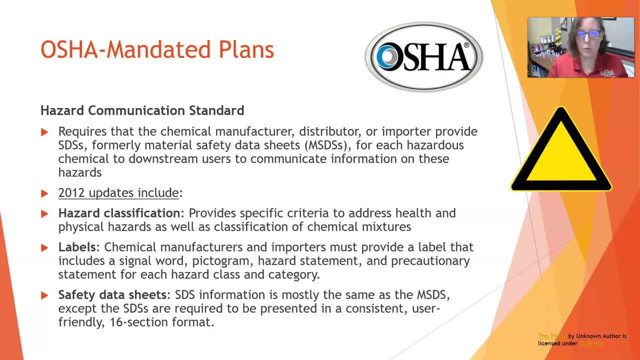 of chemicals provide safety data sheets, which were formerly known as MSDSs, which would stand for Material Safety Data Sheets, And so they provide safety data sheets, which were formerly known as MSDSs. So you have to have an SDS, a safety data sheet, for each hazardous chemical. 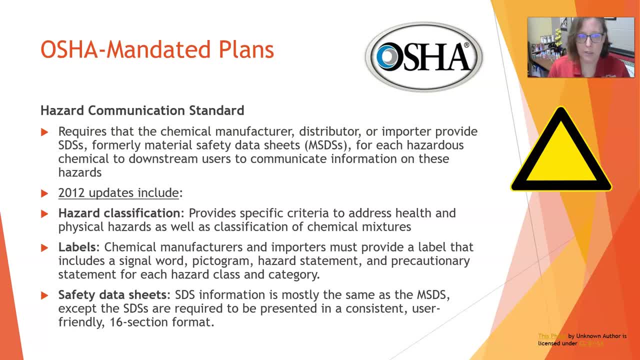 to downstream users to communicate information on these hazards. So if you handle any of these chemicals at all in your job for any reason, you have to know the information and you have to at least have access to that information and know how to protect yourself and protect your health and 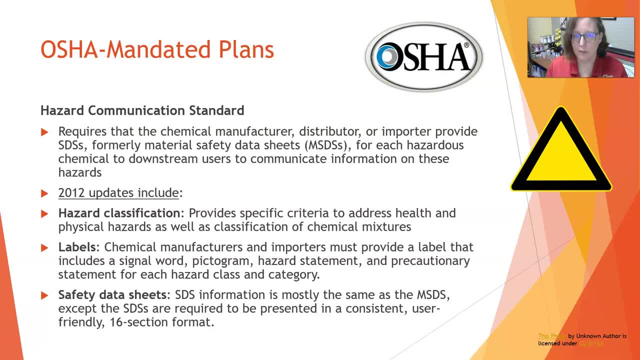 you know all of that like how to clean it up. There were some updates to the hazard communication standard in 2012.. They updated hazard classification So it provided specific criteria to address health and physical hazards. So some you know put them specifically as part of the information And then also classification of. 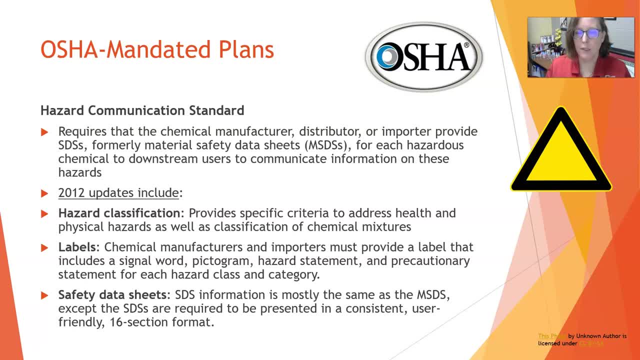 chemical mixtures, because you know, there are some chemicals that were, if each component separately would have a certain set of hazards. it would have a certain set of hazards. So maybe they don't have any hazards, but then when you mix them together they make something. 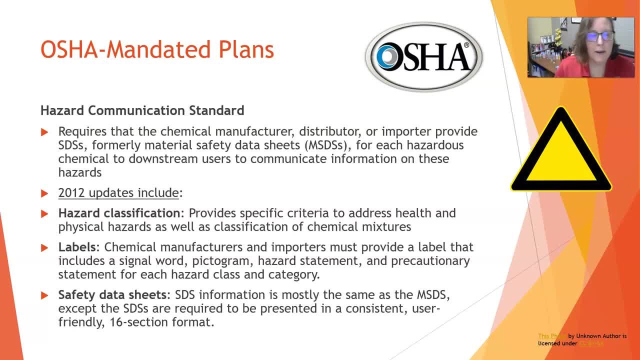 completely new that could have a whole different set of hazards, different than what the individual was before. they were combined Labels. So the chemical manufacturers and importers have to provide a label that includes a signal word, so a keyword, something that catches your attention. 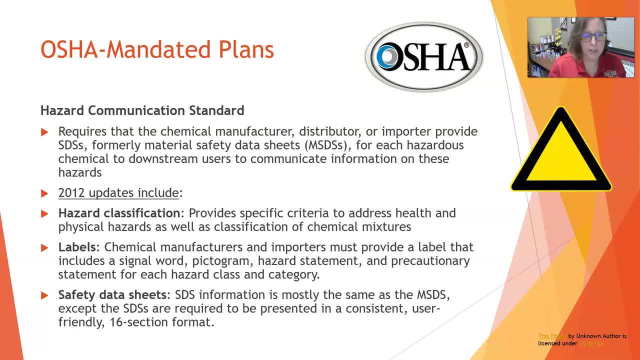 or a pictogram or hazard statement and precautionary statement for each hazard class category. So you have to be able to quickly see on that chemical: is this something that is explosive, Is this something that's a health hazard, etc. You should be able to get this. 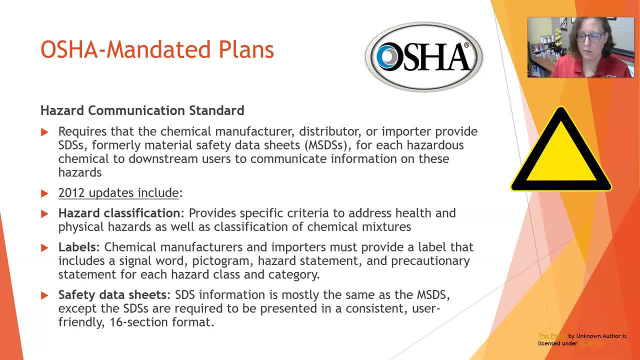 information pretty quickly if you look at the container, the label on the chemical And then, of course, the safety data sheets. The information is mostly the same as what it was when they were called MSDSs. They simply decided they wanted a consistent, user-friendly 16-section format that. 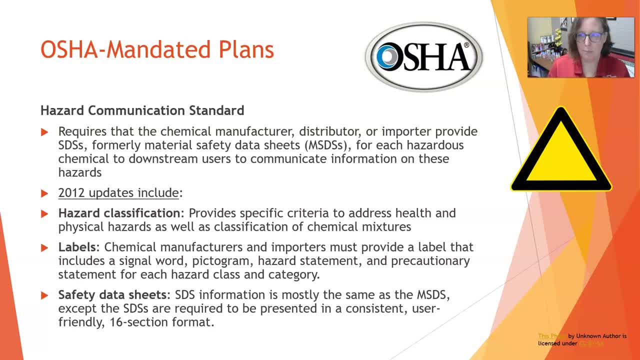 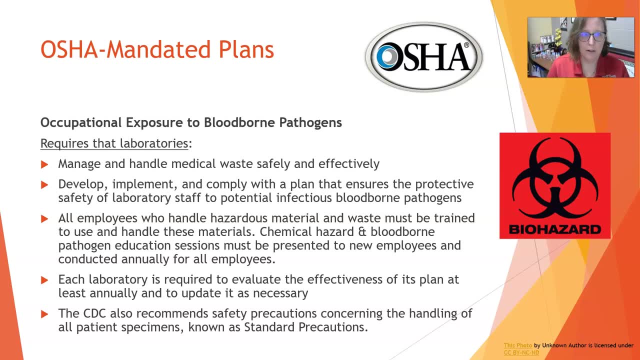 you could follow, so that you find the information in the same place, no matter where you are. And so then you have to have, of course, the occupational exposure to blood-borne pathogen standards. So that is the other protection. So you had the chemical hygiene plan. 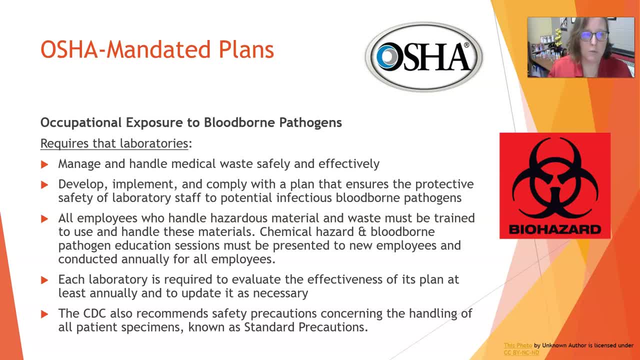 and we have an exposure plan, And so this requires that lab have to manage and handle medical waste safely and effectively. So effectively you have to have a medical waste plan, And so that also has to do with putting the right waste in the right container. So 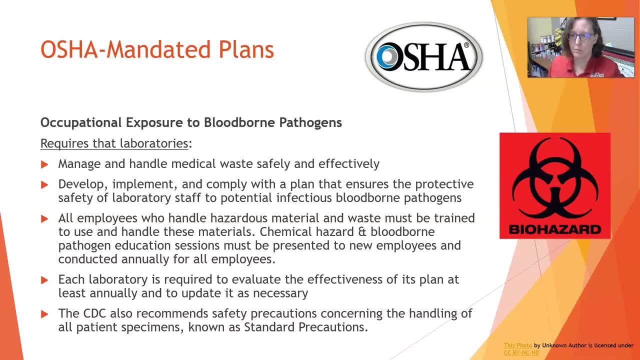 biohazards into biohazards, But then within biohazards there's also sharps, They have their own container And then you don't want to put regular trash in biohazards etc. So you know. 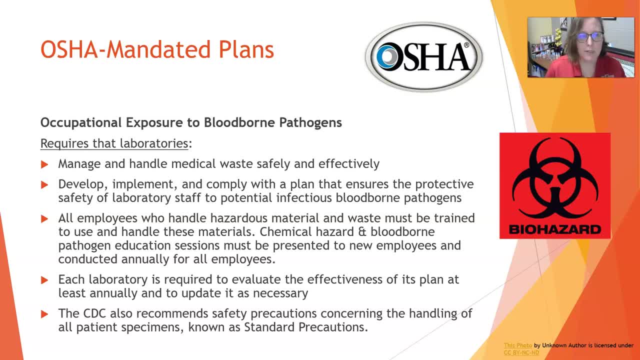 there's protocols that need to be followed. Labs also need to develop, implement and comply with a plan that ensures the protective safety of lab staff to potential infectious blood-borne pathogens. So lab have to provide you with, you know, the proper lab coats, protective gear, face shields. 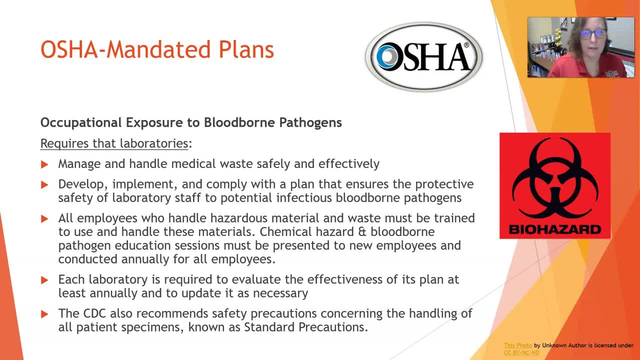 goggles, glasses, anything that you need to work safely in the lab. your employer needs to provide that All employees who handle hazardous materials and waste have to be trained to use and handle these materials. Chemical hazard and blood-borne pathogen education sessions have to be presented.